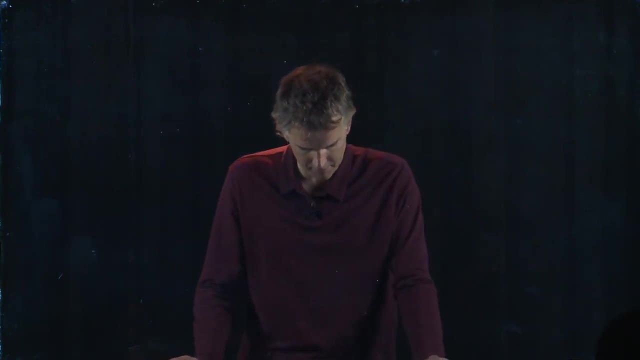 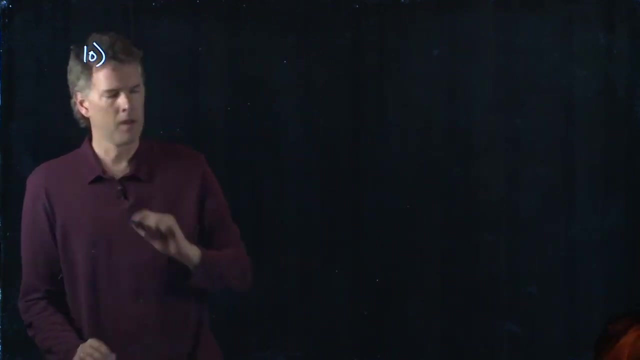 Okay, let's skip number seven. This is just more diffraction problems. I think we've done enough of those for right now. Why don't we jump ahead a little bit and look at the one that was suggested online, which is number 10.. Okay, and number 10 is a question about. 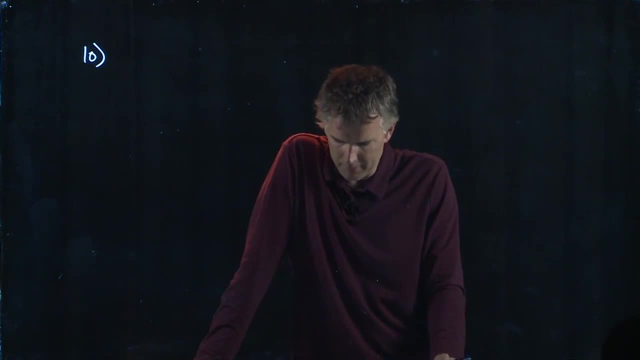 a camera. It says the focal length of the lens of a simple film camera is 40 millimeters. By what amount should the distance between the lens and the film be increased or decreased to change the focus from a person who is 25 meters from the lens to one who is four meters? 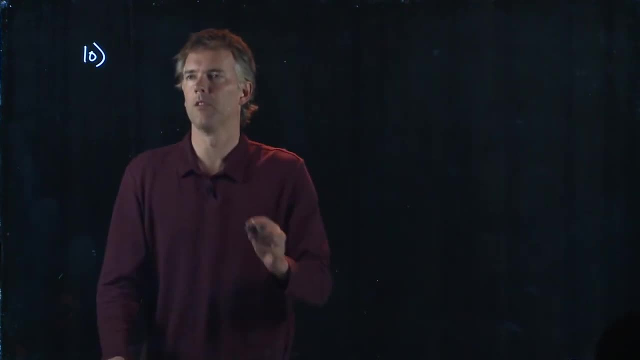 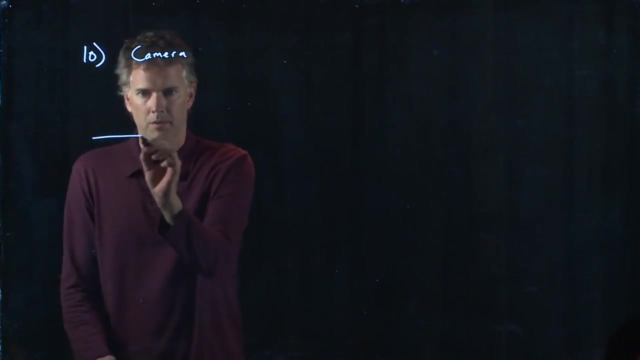 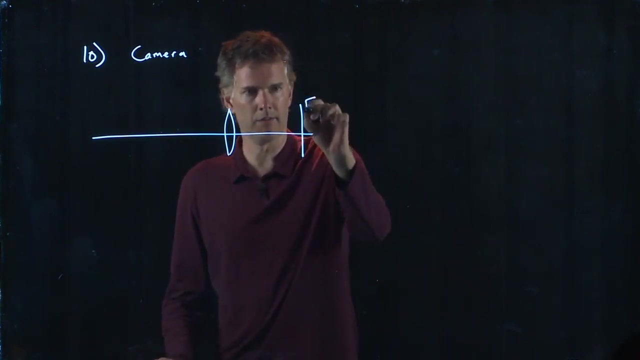 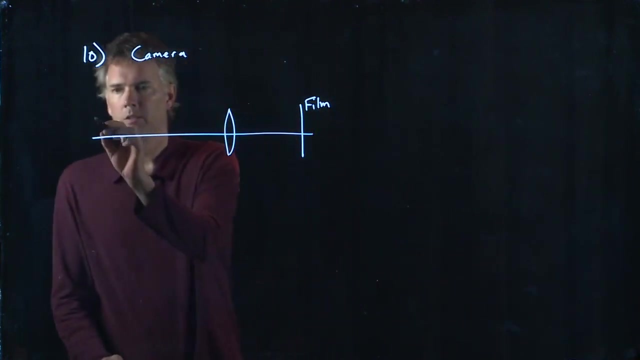 from the lens. Okay, so this is a camera problem And let's just draw a simple picture of our system. Okay, here's the lens in the camera, Here is the film plane And there is an object that is 25 meters away. 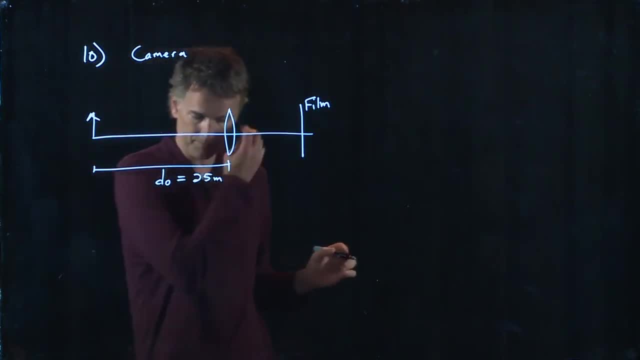 Okay, so for the first part we have 25 meters And you can follow your simple lens rules to figure out where the image is. I guess we usually draw those with solid lines right, So we'll keep them solid And therefore the image is right there. 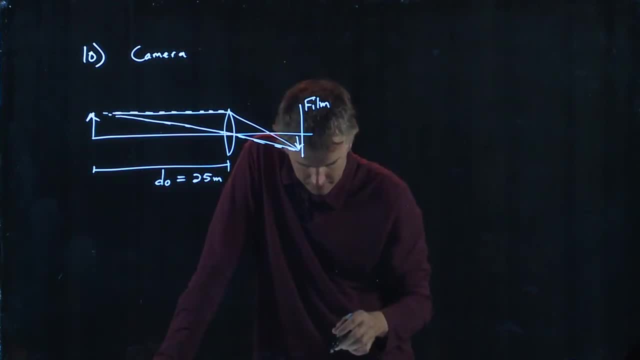 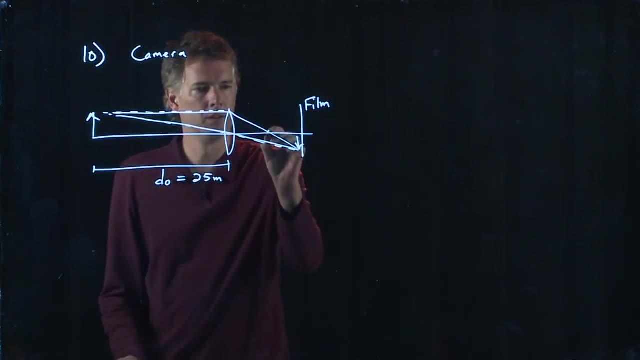 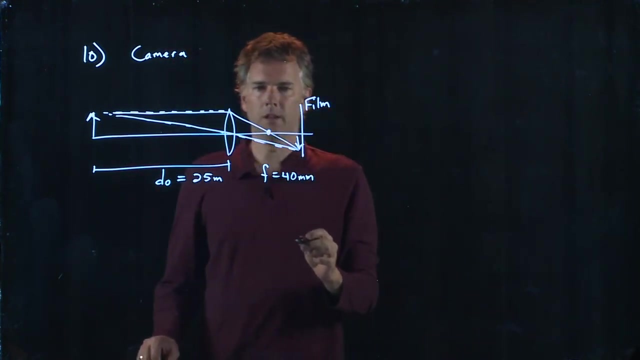 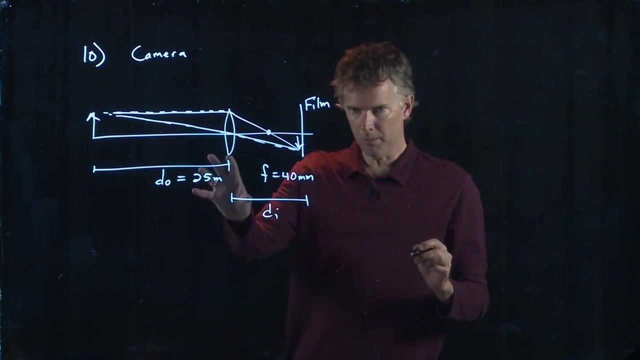 Now they tell us that the focal length of the lens in the camera is 40 millimeters. Okay, this distance here is the Socrates distance, the image distance. So with those two numbers we should be able to figure out the image. 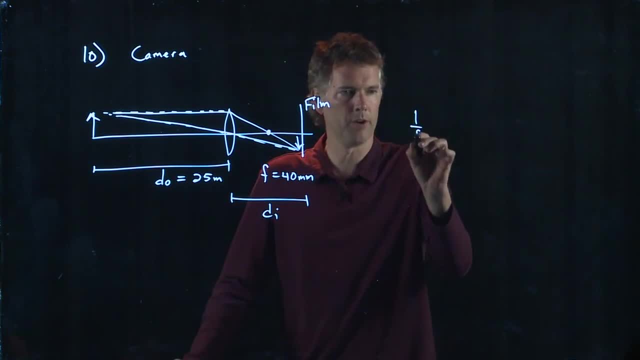 distance. in this first case, Why don't we do that? 1 over F equals 1 over DO plus 1 over DI. So let's solve this for DI. We've got 1 over DI equals 1 over F, minus 1 over. 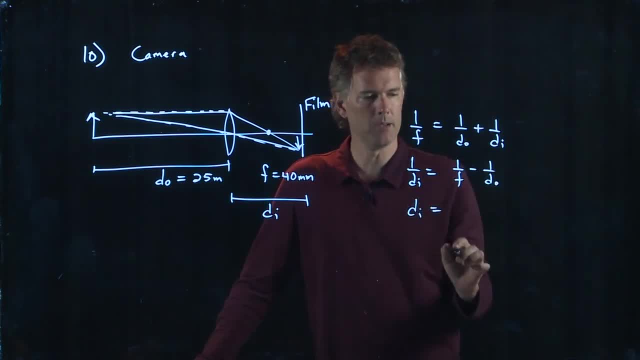 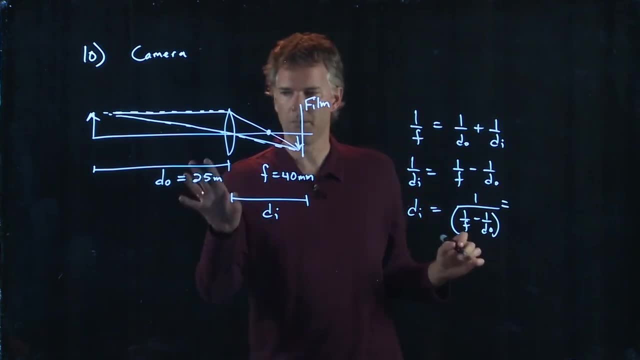 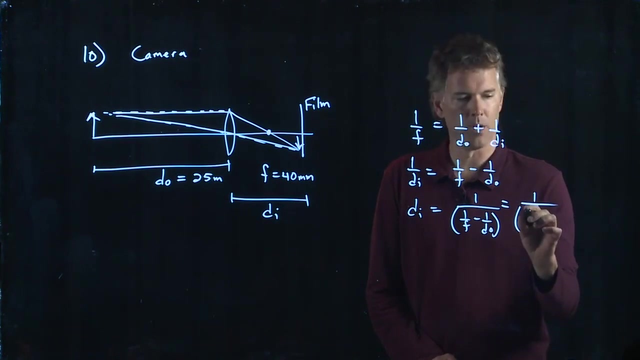 DO or DI equals 1 over that whole thing. And somebody punch in your calculator what these numbers are and let's just calculate DI to start. So 1 over F, we've got 1 over 40 millimeters. Put everything in meters, so that's 0.04.. And then DO is 25 centimeters. 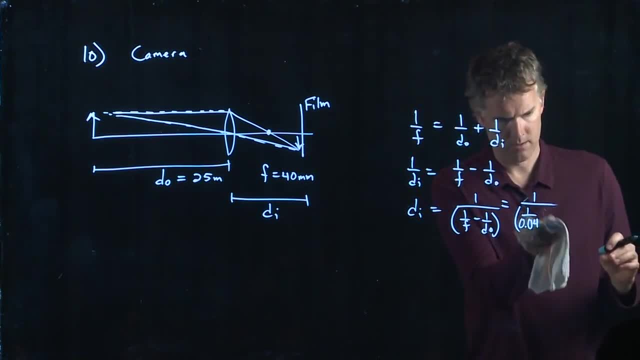 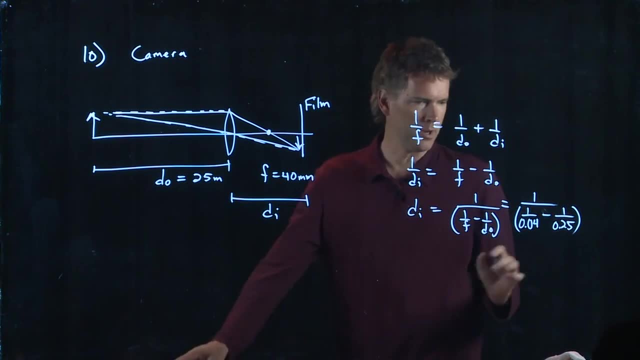 That's a minus, sorry. So we have minus 1 over 0.25.. And if you punch in those numbers, tell me what you get for DI And I can tell you it's got to be pretty close to 40 millimeters. 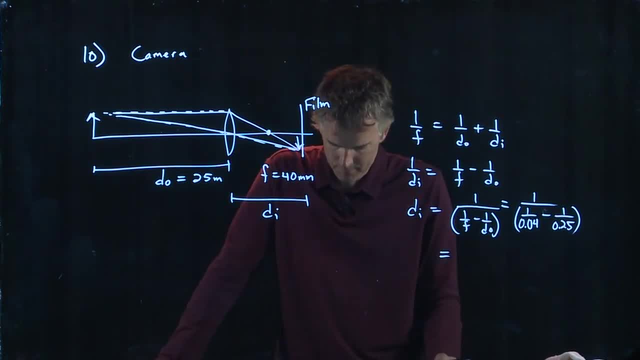 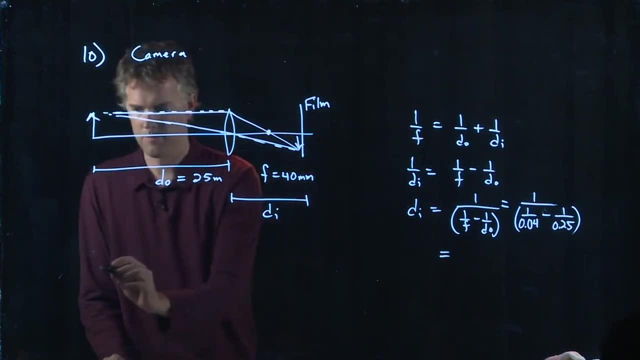 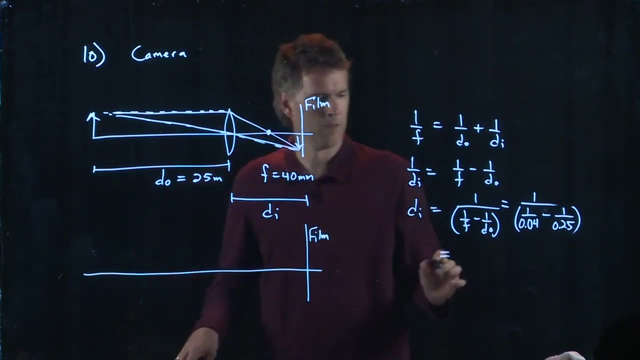 It's certainly going to be bigger than 40 millimeters, but it should be in that range: 0.01.. 0.01? That doesn't. that doesn't sound quite right to me, Because this is going to be like 20.. 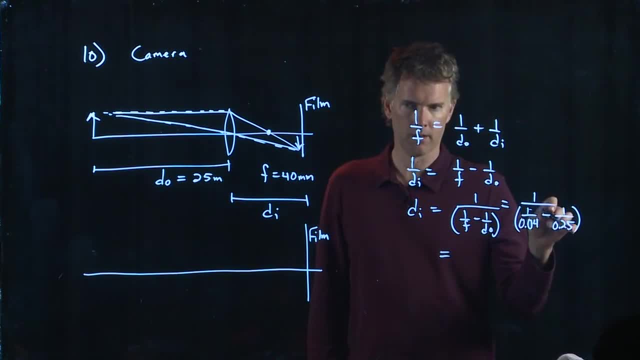 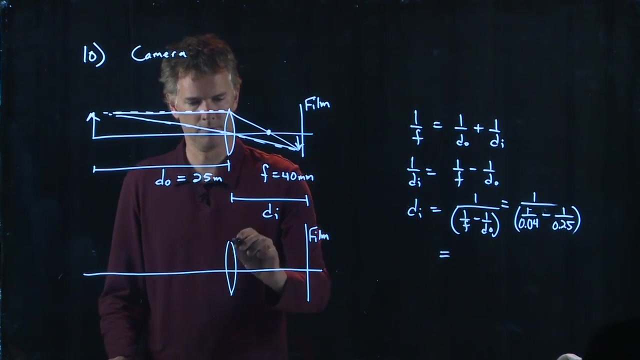 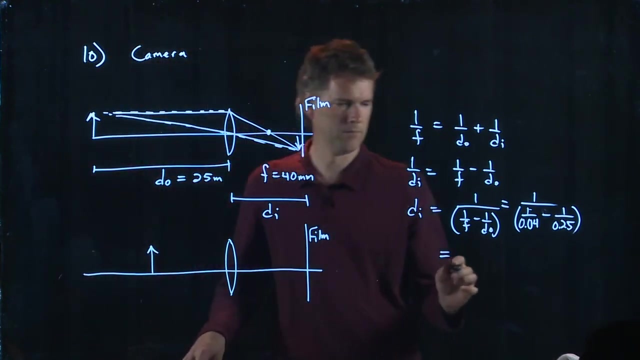 And this is 4, right? So we're going to get 20 minus 4, so that's about 16.. So 1 over 16 should be 0.1.. Anybody get an answer for that one 0.047?? 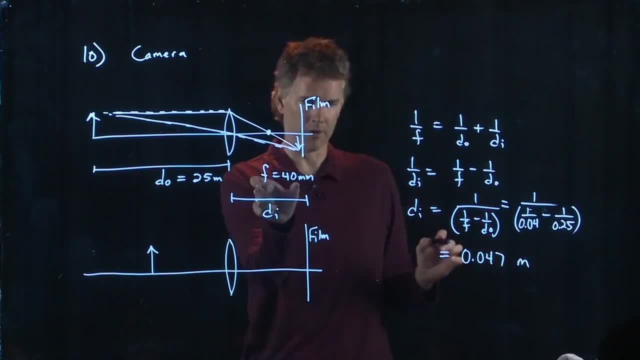 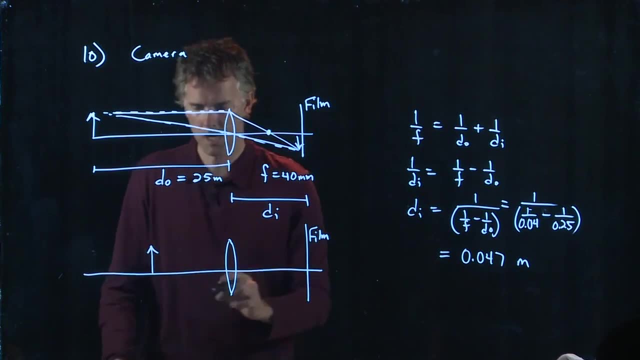 That sounds right, Okay, and that's in meters. That's certainly bigger than F, but not much bigger than F. Okay, that sounds right, Okay. so now we're going to take the object and we're going to move it much closer. 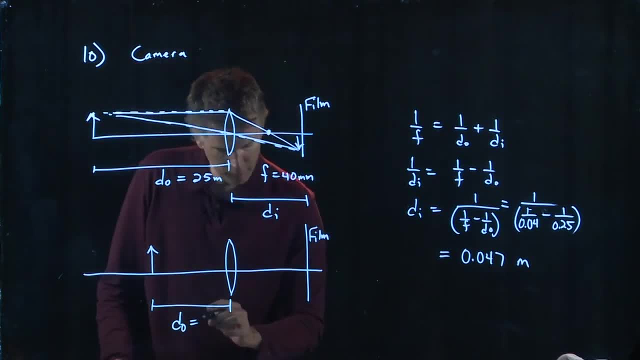 DO is now going to be four meters And we need to figure out what this image distance is going to be in this case. Okay, And what stays the same, of course, is the focal length of the lens. So if we had left the lens exactly where it was and I brought that object in, would the image: 0.12.. 0.13.. 0.15.. 0.16.. 0.17.. 0.19., 0.20., 0.20., 0.29.. 0.30.. 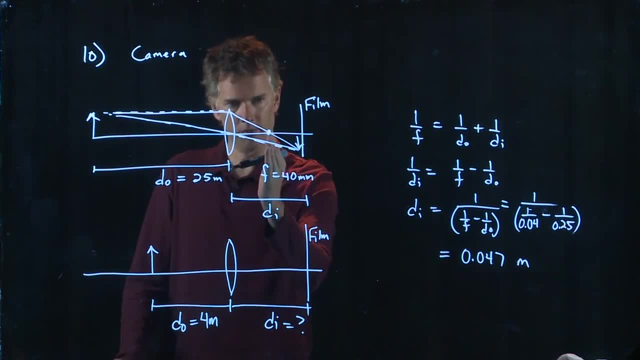 0.40.. 0.24.. 0.4.. 0.33.. 0.55.. 0.さん. move closer to the focus or further away from the focus? it would, in fact, move further away from the focus. okay, so you still follow your lens rules, but the 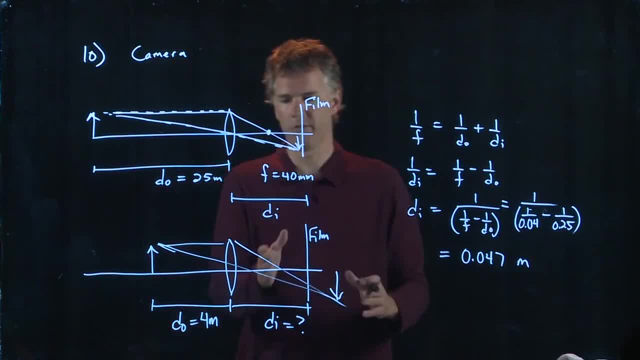 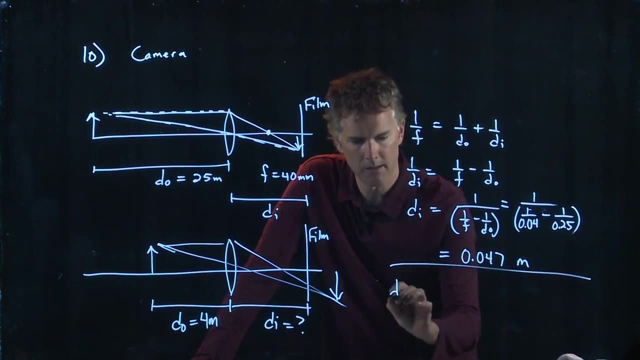 image would be out here, and so, in fact, I need to move that lens further away from the film. but since they give us all those numbers, we can just calculate it right. we know di. in this case, di is going to be this thing: 1 over 1 over F. 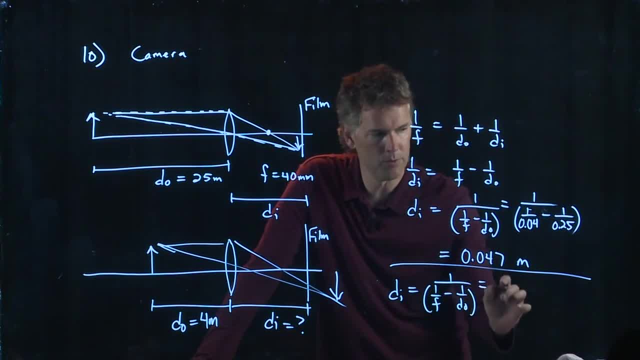 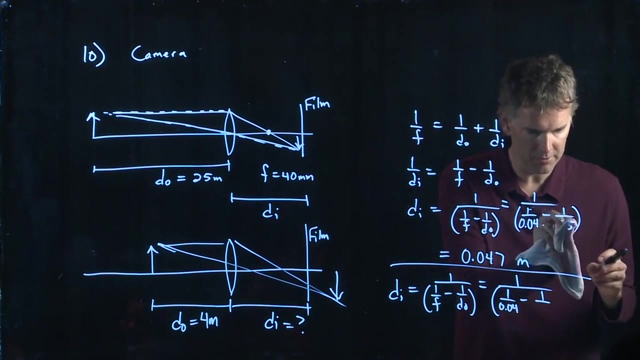 minus 1 over do, but we have new numbers for do, so we have 1 over 0.04 minus 1 over. I think we messed this up, didn't we? yeah, yeah, that's. I thought that was centimeters. that's not centimeters, that's meters. this was not 0.25, this was. 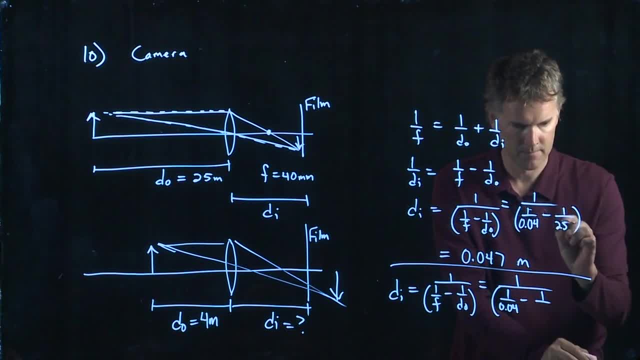 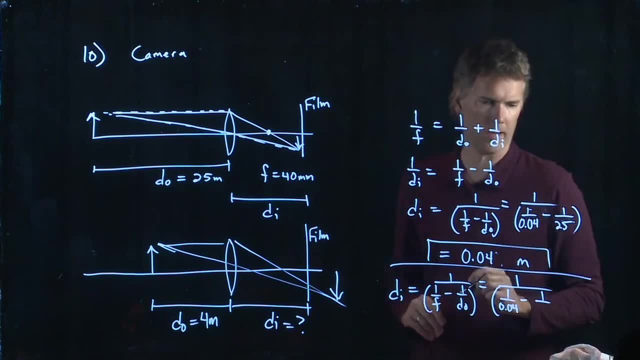 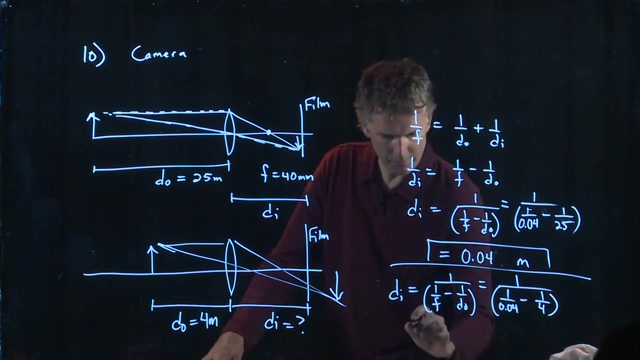 25, in which case this number is going to be basically 0.4. double-check me on that one. there might be one more digit after it, but it's basically zero point zero four. okay, and now, if you do this, tell me what you get. yes, this is good practice for tomorrow: punching things into your calculator. 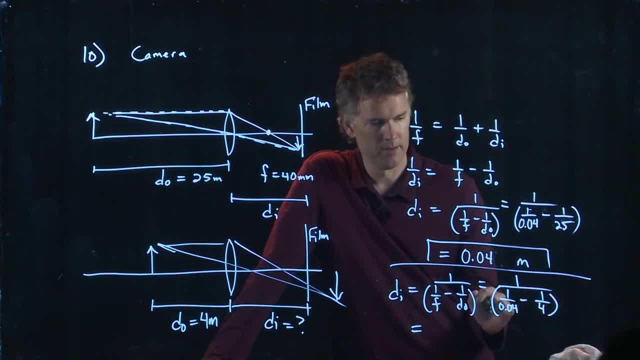 anybody else bring their calculator with them. for the first one, you got 0.0, 40, .0, 4, and what do you get on the first one? Okay, so if I take the difference between those two, what do I get? Something really small right.